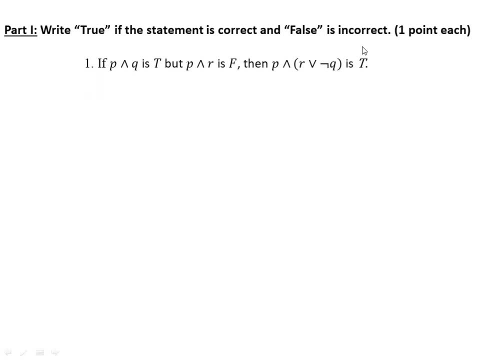 each question has one point. question number one says that if p and q is true, but p and r is false, then p and r or negation q is true. now to determine whether or to say this is true or false, let us check here from this: p and q is true, then we obtain what p is true. 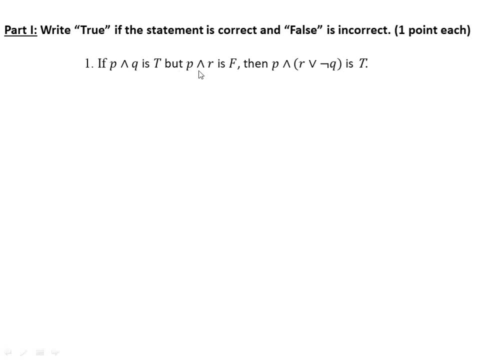 q is true, therefore p and q are. both are true. and here we say that p and r is false, p and r from this, p is true, therefore true, and r is false, then simply the values of r should be what which is false, because p is true, therefore p, q, p and q are true and we 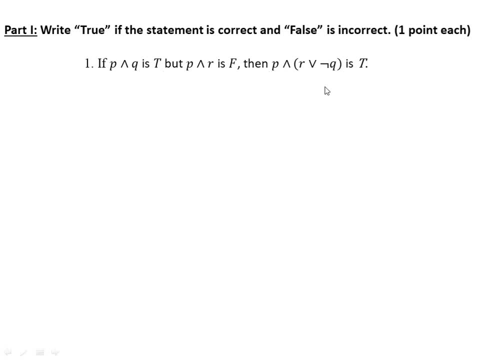 obtain r is false, then we can determine the truth value for this. therefore p and r or negation q become states here. p is true, therefore p and q are false and we obtain r is false. p is true, true and r is false or negation q. negation q is false, therefore false. or 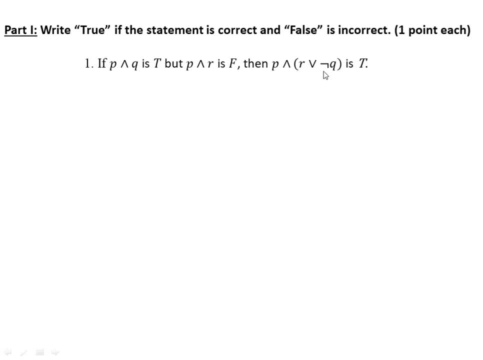 false, which is false, therefore true and false, which is false, therefore this has what which is false. number two: the compound statement p, bi implies q, bi implies q & q implies p is tautology. yes, this is true, because this p and q is found and these two things are true, and therefore n minus c is true, since in song that the lowest 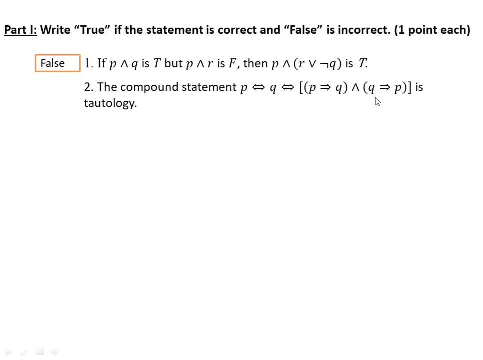 value of q is written: cos p minus c is always sin i. This parallel terms, the geezer, form a covalent result. this p implies q and q implies p. therefore, this compound statement is, which is totally true. therefore, this is true. number three, for any sets a and b. if a without b is a, then 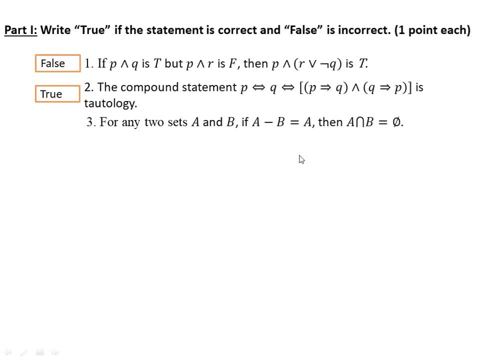 a intersection between no for a without b, or a set which contains an element only in a, not in b, which is a. therefore, and this means what? and b has not any intersections. therefore, this is true number four, let the universal sets you is a real number, then. negation of there exists x, x squared. 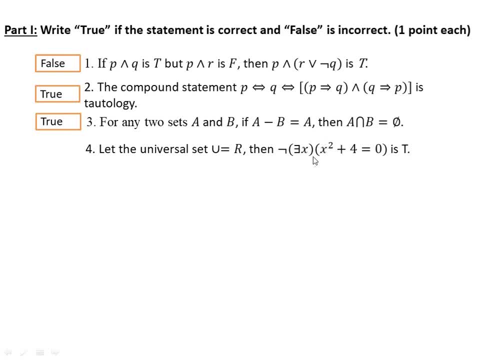 plus four is equal to zero. is true. now to determine this. let us we can find this. what means this negation of there exists x? x squared plus four is equal to zero means what for every x? x squared plus four is different from zero? therefore, for any x from a real number, 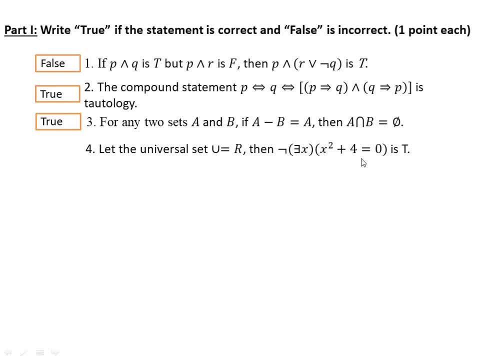 x squared plus four is what not only nodes always give us zero. therefore, x plus four is not equal to zero for any x in a real number. therefore, this is what which is true. before this statement has to survive. the statement is which is true. part two give. 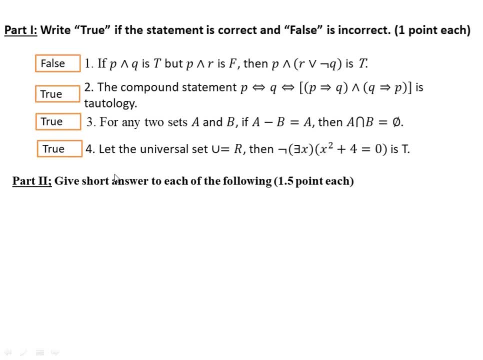 short answer to each of the following. each of those following questions has 1.5 number. five says that let the universal set u is integer, which is z, and let a of x say that x is an even integer. o of x, x is an odd integer. then the truth values of a: there exist x. 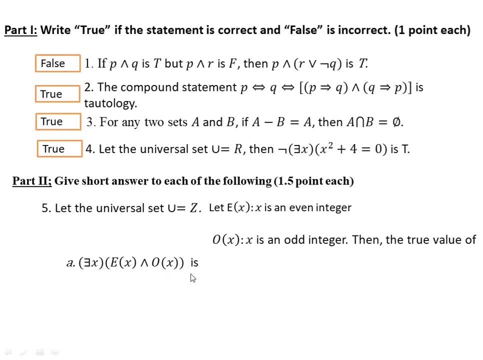 e of x and o of x is dash now here, since a of x is 11 or o of x is, which is out. therefore, so that there exists an x form integers, which is both even and odd. therefore, this is what which is false. therefore, there is no a e integers, which is both odd and ever. therefore, this is which is false. 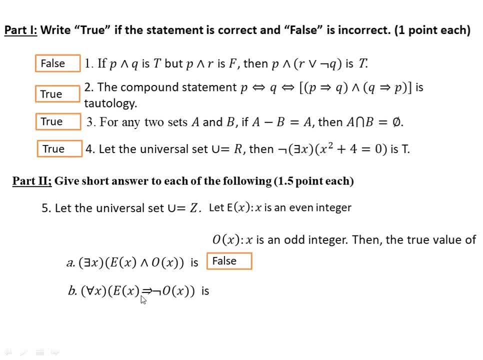 b. for every x there exists x, then of x implies a conditional of o x. what is the integration for x? pagination of o of x is which is a of x. that means even, therefore, that's for every x, a of x implies a of x, which is. 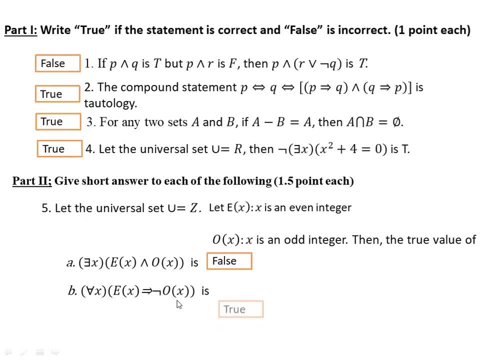 because it the number implies that the number of chatting with us, which is too number 6.. relates the statement p, q, r and a is to e, to for f, i, as for n, am, y, a and m? nC. but yes, that implies that n and is also to let's the statement p q R for x. as i had expected, P Q R for x and u is true. number six relates the statement p Q R for x and L N xe psyche. pq, Q, R and l? x are taxi K by n? Ne inner space, plus constant from the denke shape of G and if the number implies that, if a number gives us which is true in it. 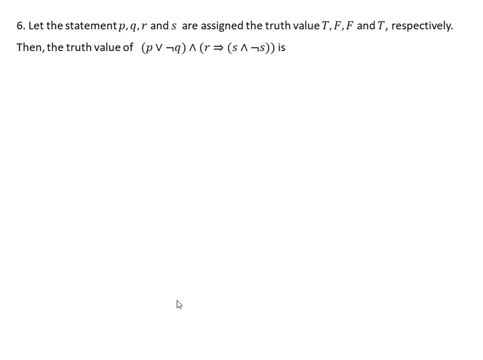 very important that you solve the equation and that it should be in the dry~. Q, R and S are assigned the truth values true, false, false and true respectively. It means that the truth values for P is true, Q is false, R is false and S is true. 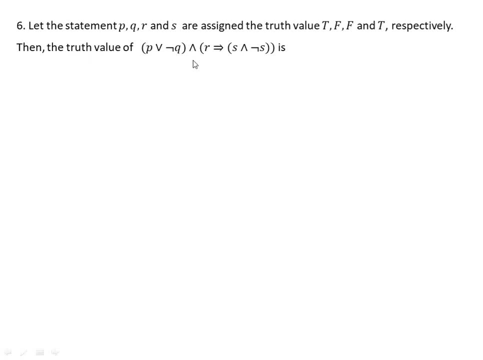 Then we can determine the truth values for these compound propositions. Therefore, to determine the truth values for this here, P is what True And Q is which is false. therefore, negation Q is which is true. therefore, this means what P is true, therefore true, or N is truth values which is true, therefore this has true. 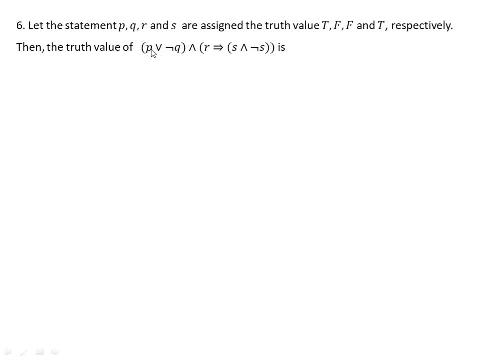 This statement has truth values, which means true or true is, which is true. therefore, this is true And let us confirm this here. R implies S and the negation of S, S and the negation of S means what, Since S is true. 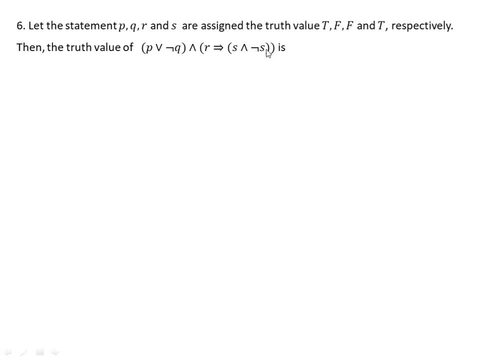 Negation of S is false, therefore true and false is, which is false. Here, R is, which is false, therefore, False implies false, which is false. but this is true. therefore, true and false. No, true and the true, this is true. 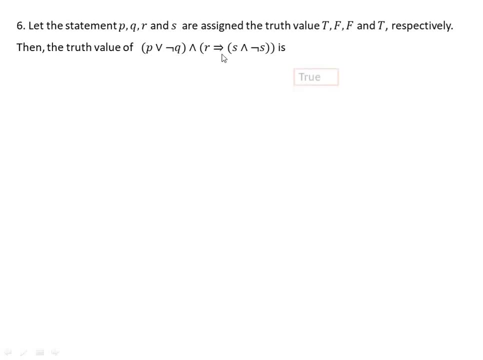 True and the true, which is true, therefore, this statement has, is what True Number 7.. Let set A is given us, the set containing an element 1, the set containing 2,, 3, and 4. Then the number of subset of set A is dash. 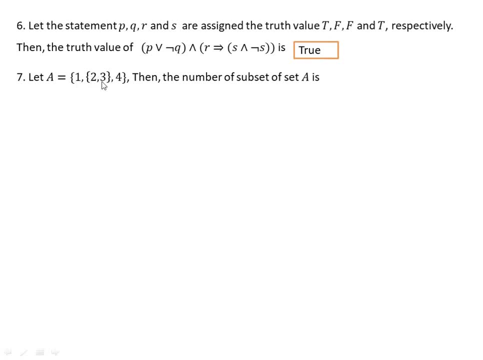 The elements are this set A has. Now, this set A has what? 3 elements. Therefore, using the formula, the number of subset of- if A has infinite number of elements, then also the number of subset for given set A is what. 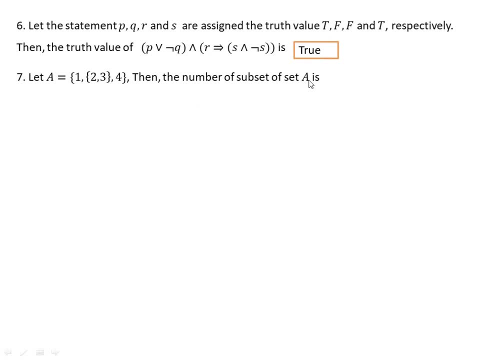 To the power of N- Therefore here R, N is 3, then to the power of 3, which is 8.. Number 8.. Given the statement, If a number is not positive, then it is less than 0. Then A the converse. what is the converse for this statement? 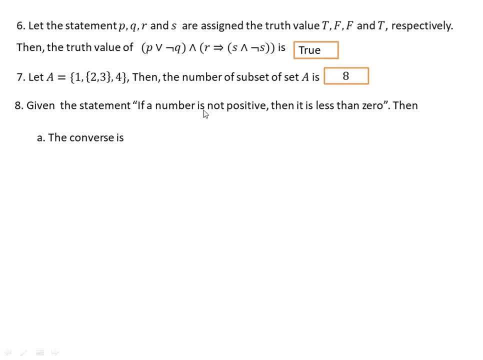 Now, here the converse means simply by interesting, or writes the hypothesis as conclusions and the conclusions as hypothesis. Therefore here, if a number is not positive, then it is less than 0. Its converse is, what If a number is less than 0?? 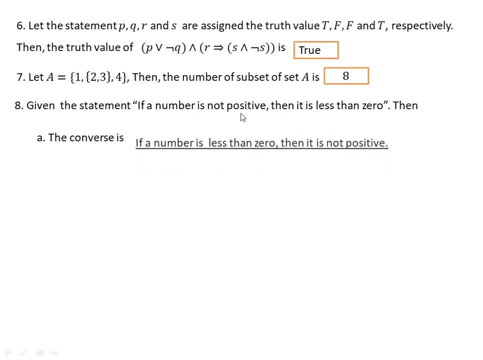 Then it is not positive. It is like this: If a number is less than 0, then it is not positive. B- what is the inverse? Now, the inverse for this statement is what Simply find the negatifs for the given statement. 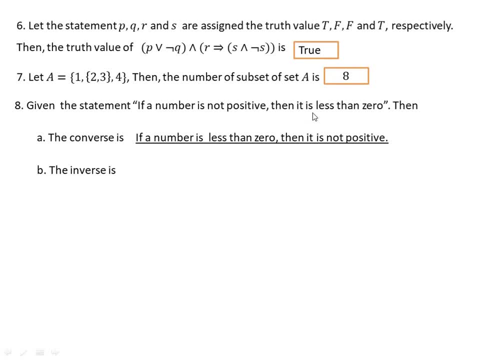 That means, if a number is positive, then it is not less than 0.. Or if a number is positive, Then it is not positive, Then it is positive, Then it is not negative, greater than or equal to zero before. if a number is positive, then it is greater. 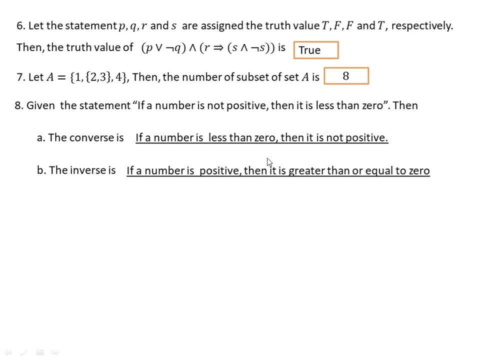 than or equal to zero, or if a number is positive, then it is not less than zero. see the contrapositive. the contrapositive is simply the negation of converse. that means, if a number is not less than zero, that it is positive, or if a number is 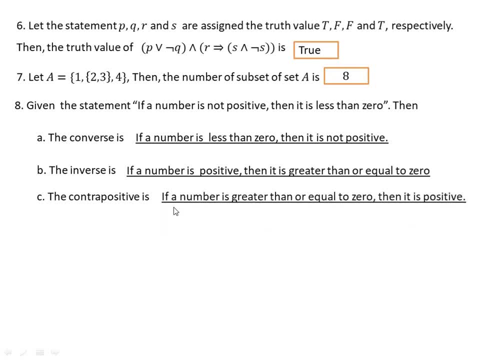 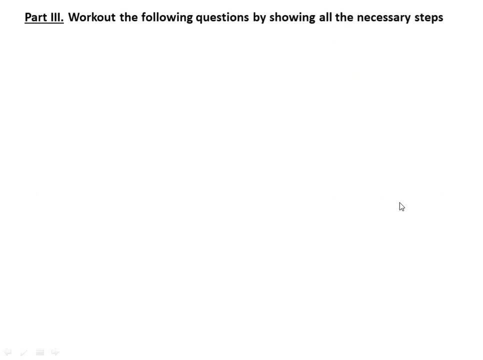 greater than or equal to 0 is it is positive, which is given here, if a number is greater than 0 or equal to zero. if the number is greater than or equal to zero, then it is positive. Part 3: work out. work out the following questions by showing: 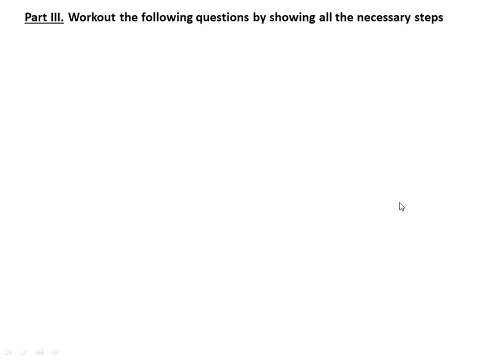 all your answers 今日. all your answers. the necessary steps, number nine, show that the following argument form is valid or not. now the given argument is given here: P implies Q, Q implies R, negation Q. those are as hypothesis or the premises, and the conclusion is negation of R. so 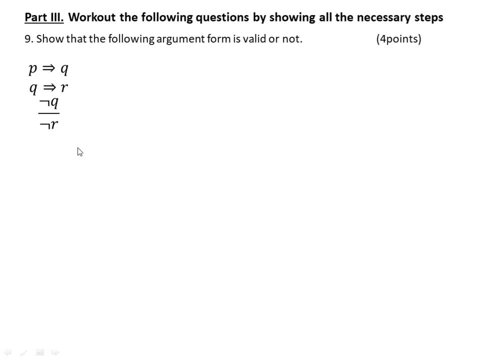 now for simplicity, let us check the validity of this given argument using or constructing the first ever now, the travel for this view that my given like this, since here we have three propositions. she speak in plays therefore eight possible trust-value combinations, and P, Q, R and P. 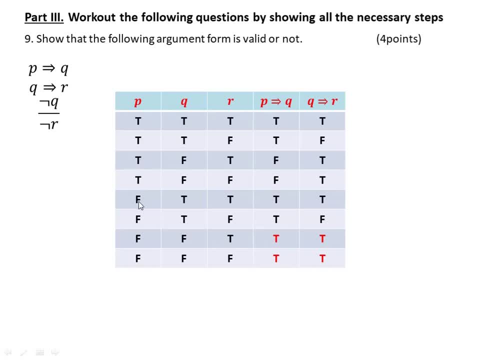 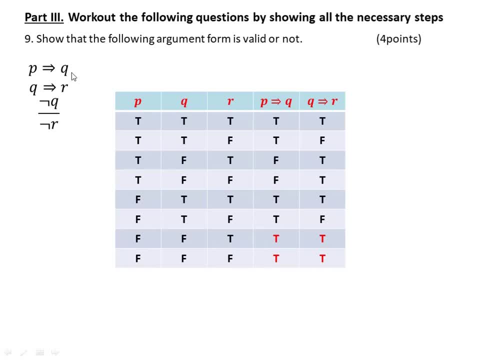 Then next we can determine: P implies Q. Now, P implies Q is always false. if P is true and Q is false, Therefore P implies Q has possible through's value, has true's value, which is true, true, false, false, true, true, true, true. 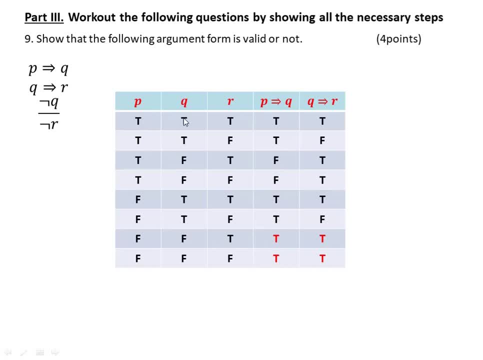 because here, true implies true is always true, which is true. Q implies r is false, even though Q is true and r is false. therefore, Q implies r has value, like this the definitions. now, using this truth table, we can determine whether the given argument is valid or. 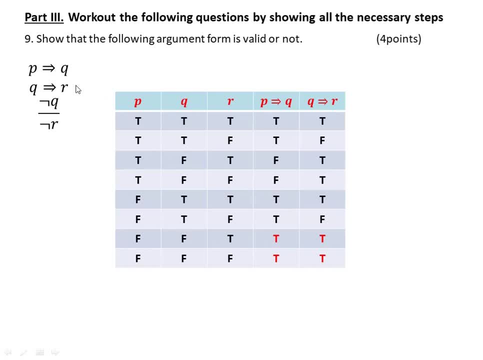 invalid now here. so i told you that p implies q, q implies r and the negation q are premises. then from this truth table we can find where those p implies q, q implies r and negation q are true. then corresponding through those premises we can determine it is conclusions or 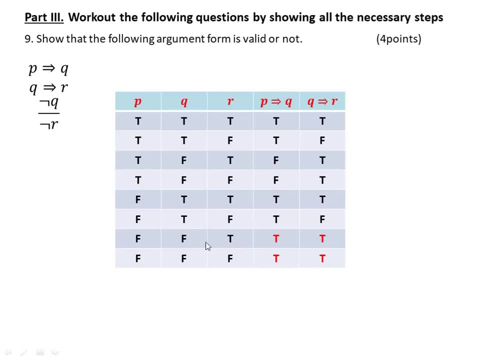 negation now here, only in eighth, in seventh, in seventh and eighth row, those the, uh sorry, here we have, can determine the decision q based on q, because q was: if q is true, true, false, false, false, false, then negation q is false, false, true, true, false, false, true, true, then negation r is. 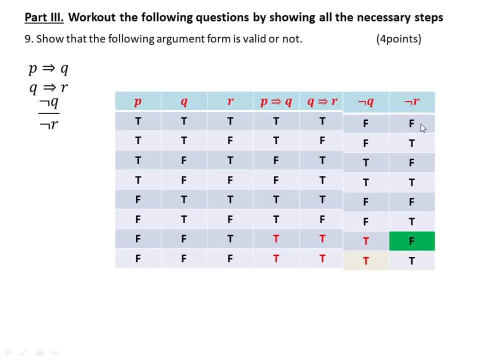 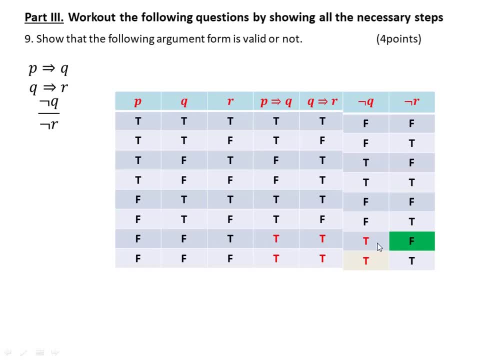 in both column row seven and eight, the premise has truth value, which is true, but in seven zero, the calculation, which is negation r, is false. as a result, the given argument is: which is invalid. like this, the premises: p implies q, q implies r and the negation 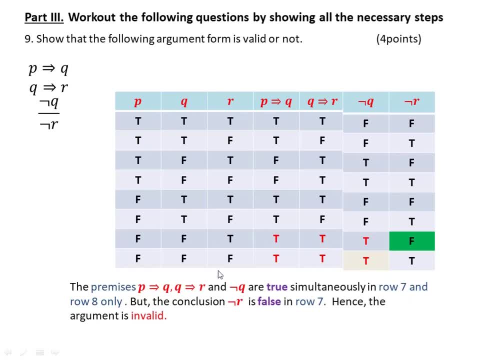 q are true simultaneously in row seven and row eight here, but the conclusions, which is a negation, r is which is false in row seven. hence the given argument is which is invalid. there are. we can also. we can take this validity using the formal or using inference rule, or using 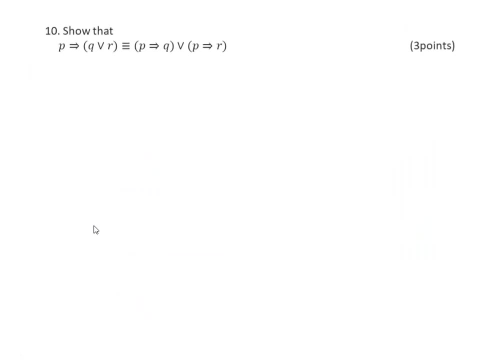 formal definitions n number eight, show that p implies q or r is equivalent to p implies q or p implies r. now we, for example, because we can show this using our constracted ruse table or otherwise, you can prove using formal loop. that means by noting that by using the definitions for p implies q, since 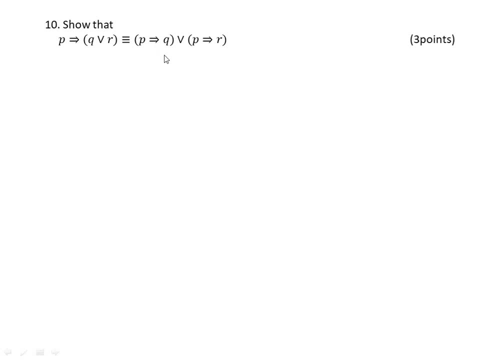 p implies q is equivalent to this negation p or q and using that difference that we hear this also by the definition in the form of p plus q, p implies q or r is also equivalent with what negation p or q or r. and since p implies q, is also negation p or q. 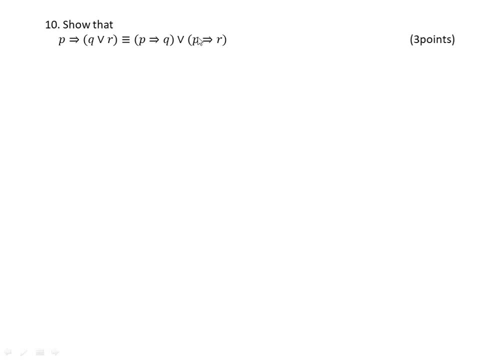 and this p implies r is also equivalent with negation p or r. then by using constructing or by using the associative law for these junctions, we can prove in simple head, but in other case let us we prove this or we show this by constructing through's table. 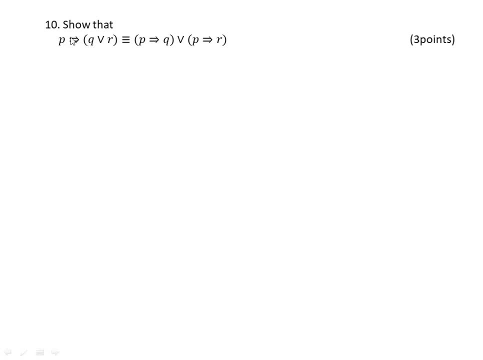 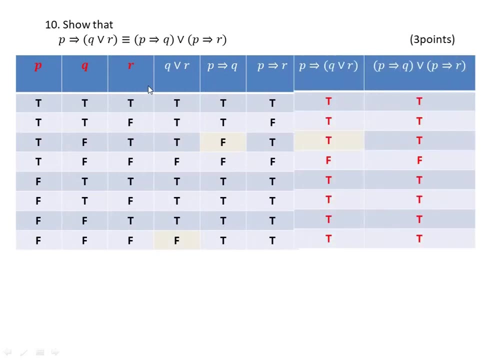 now here, since we have three propositions, say p, q and r, therefore they have hat's. eight possible combinations through's tables are given here. now, here, since we have p, q and r, p has possible truth value which is true, true, true, false, false, false, false. when the q has true, true, false, false, true, true, false, false. 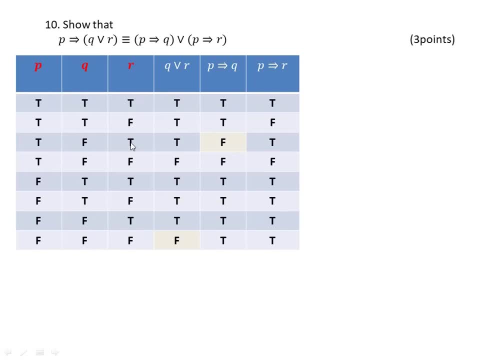 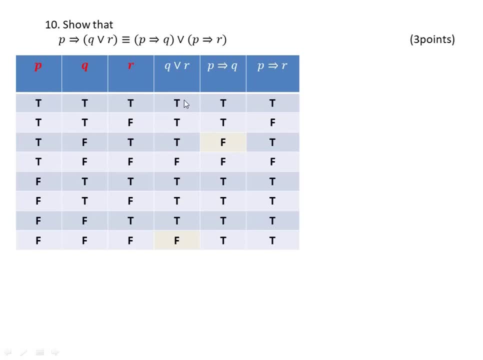 otherwise q or r, as there is value, true true force, true true true force and the p implies q has. since p implies q is false if p is true and the q is false otherwise. p implies r has also truth value, which is false if p true, q is, r is false otherwise. therefore, p implies r implies p implies r has true's value. 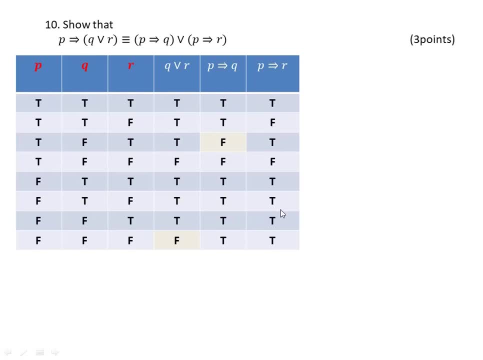 true, false, true, false, true, true, true, true. then let us determine this: p implies q or r. and finally, p implies q or p implies r. now, p implies q or r has true's value: true, true, true, false, true, true, true. and this p implies q or p implies r. here we have p implies q and the. 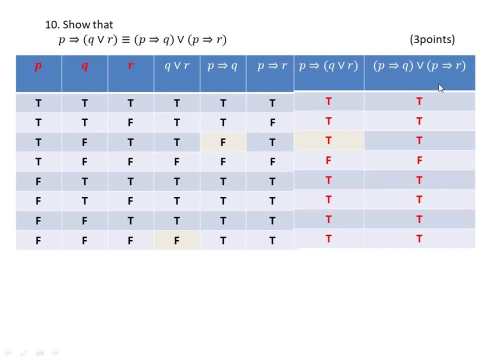 p implies r, then we can join by these junctions, which is off. therefore, this has true's value, which is false. if both p implies q and p implies r has false, false, otherwise. so therefore, this has true's value, which is true, true, true, false, true, true, true, true. then we can observe that 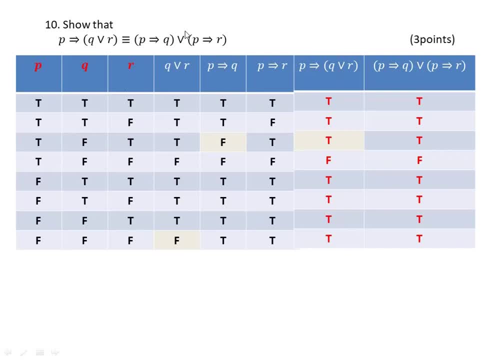 this: if this is column 1, column 2, column 3, column 4, column 5, column 6, column 7,, column 8.. Therefore, from column 7 and column 8, those compound propositions has identical terms. as a result, Those compound propositions are equivalent. 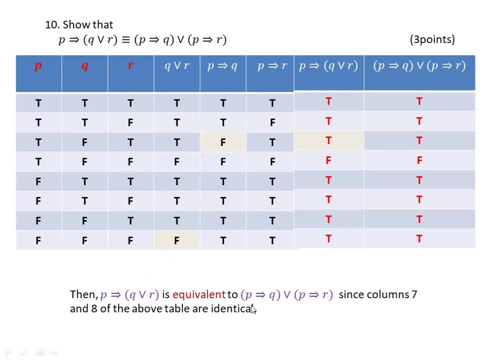 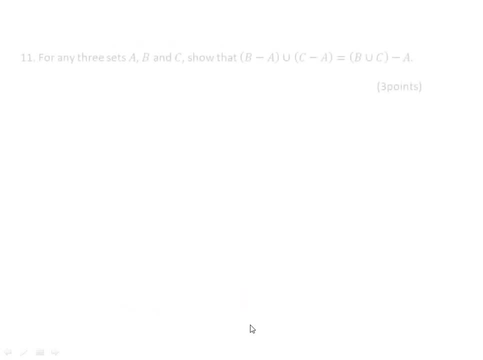 Oh, that means then P implies Q or R is equivalent to P implies Q or P implies R. since column 7 and column 8 of the above table are not identical, Number 11. For any three sets- R, P and C- show that B without A or C without A is equal. 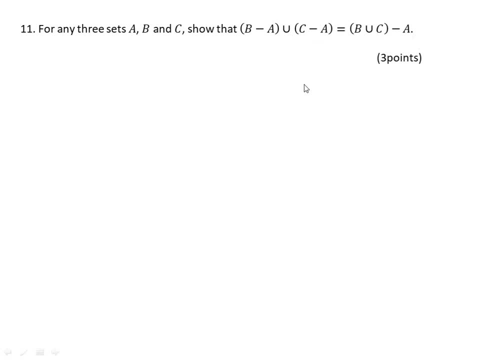 to B, union C without F. Now here let us we start from this, from the left-hand side of the solutions. This has three points. And now let us start from the right-hand side. And now let us start from the left-hand side. 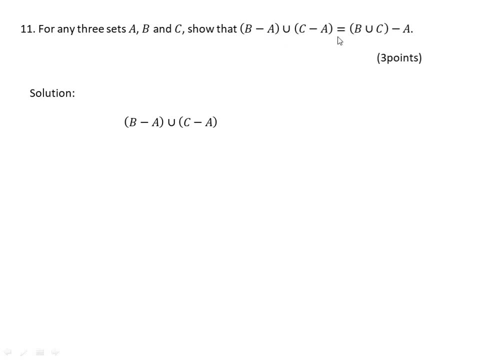 And now let us start from the right-hand side. And now let us start from the right-hand side. Let us start from this left-hand side. P without A or C without A? Then what means B without A and what is C without A? Now, P without A is the same as what? B intersections A complement. 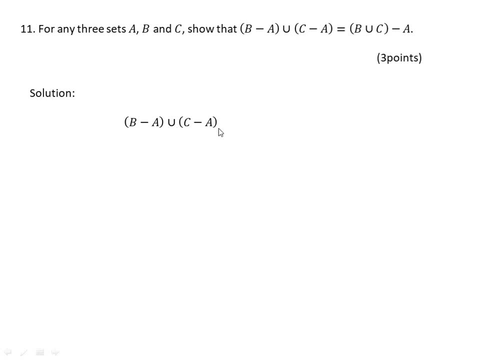 And C without A is the same as C, C intersections A complement. Therefore, this is equal to what? B intersections A complement, or union C intersections A complement. Dear, all here, we have A complement as a common, isn't it? 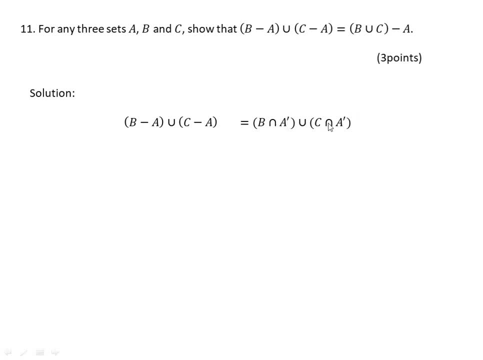 So common word here, not only A complement, intersections A complement. intersections A complement are common. Therefore let us take this common word here. If we take intersections A compliments as a common word, then we left what Б, union, C, intersections A complement. 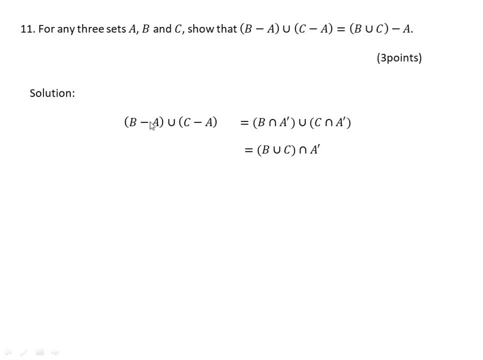 Again, as I told you that, since B without A is the same as interviews, a compliment, which that means the intersections, a compliment, the same as B without A. Therefore, B union C intersection complement is the same as what B union C without a, which is gives like it like. 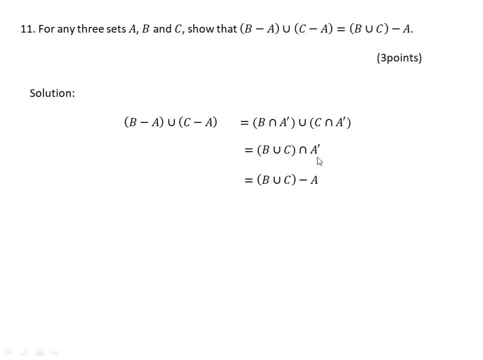 this B union C without a, isn't it, therefore, which is proved so? thanks for watching my video, but anybody who subscribed my video don't forget again to like it, my video, thanks.